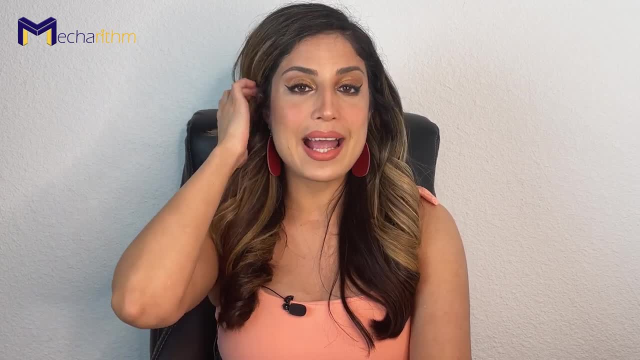 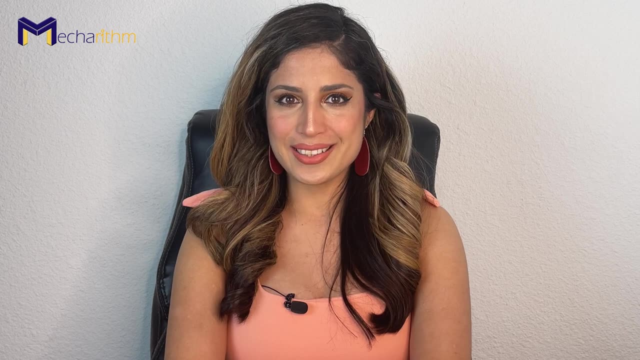 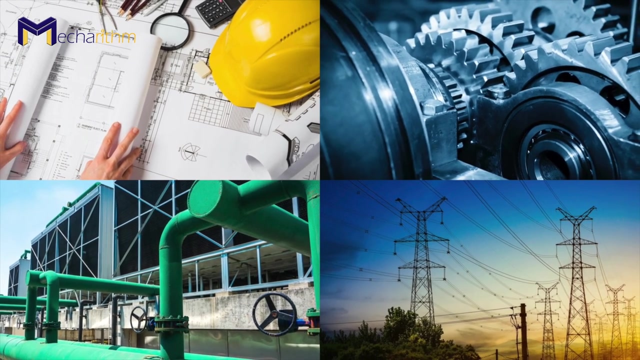 on a lesson. Also, let's help other people to get access to robotics and mechatronics lessons by sharing this lesson with them. I sincerely thank you for your attention and, without further ado, let's get it started. Mechanical engineering, electrical engineering, civil engineering. 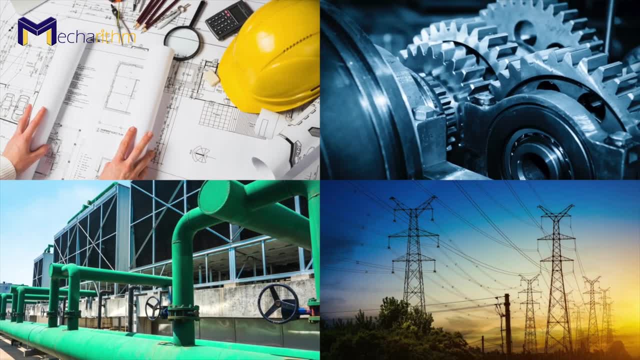 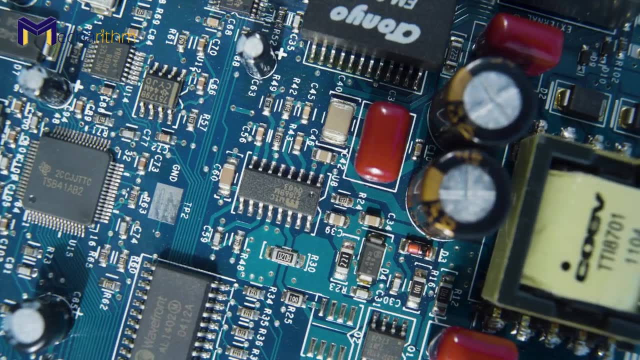 and chemical engineering are all part of mechatronics. They are all part of mechatronics. Mechanical engineering were the primary engineering disciplines of the 20th century, but a breakthrough in semiconductor electronics and the use of integrated circuits and computers changed the boundaries of traditional engineering disciplines. 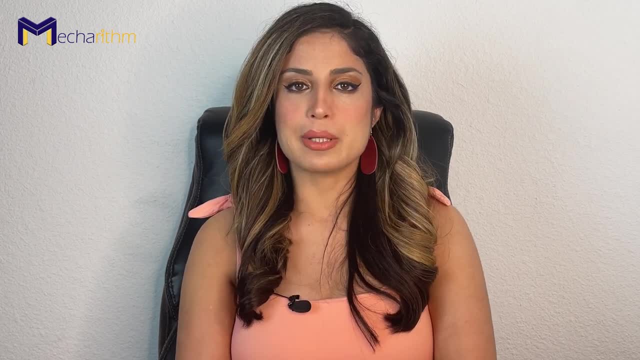 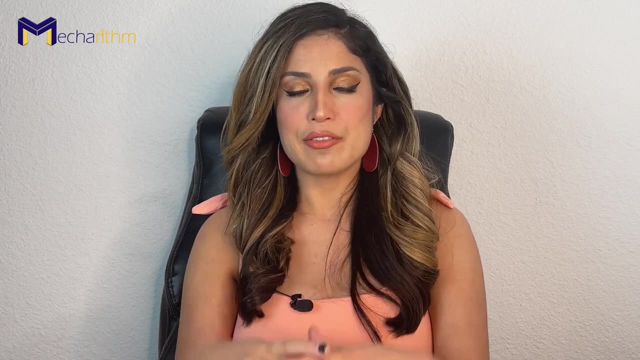 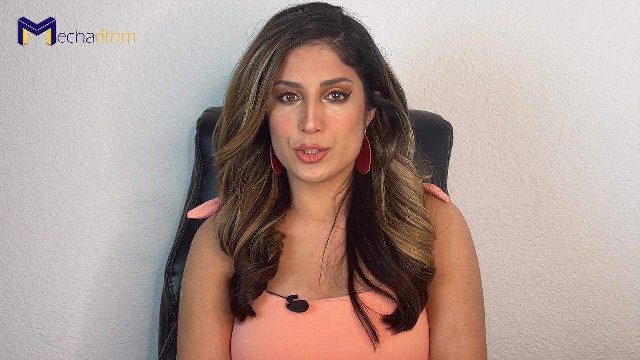 Mechatronics is a field of study that combines electronics and mechanical components with modern controls and microprocessors. As a matter of fact, every newly designed engineering product can be considered to be a mechatronics system. The word mechatronics was coined in Japan in the 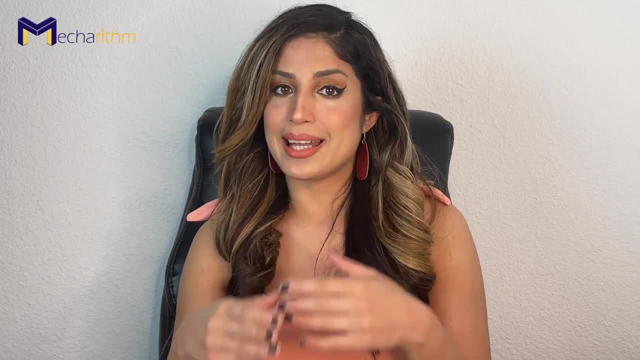 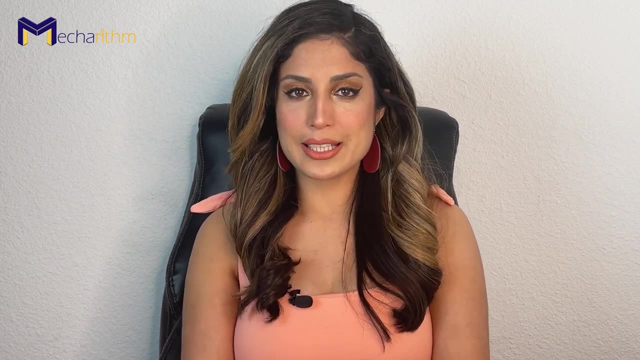 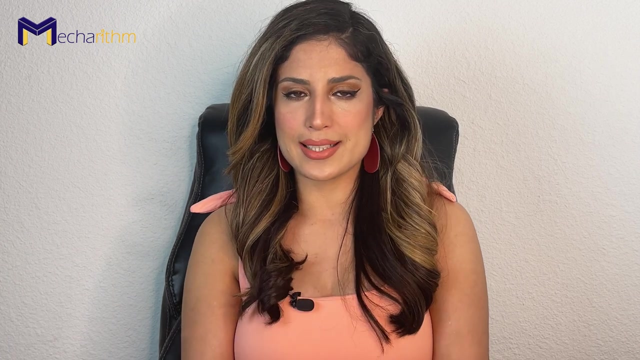 1960s spread through Europe and then eventually took off in the United States. A mechatronics system is sometimes called a smart device because it combines logic, computation and feedback into a very sophisticated and complex design to simulate human thinking process. Now the question. 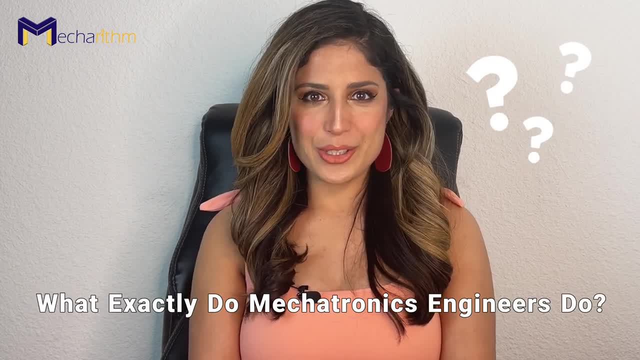 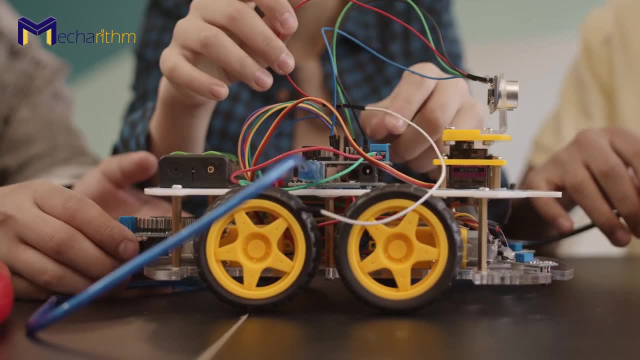 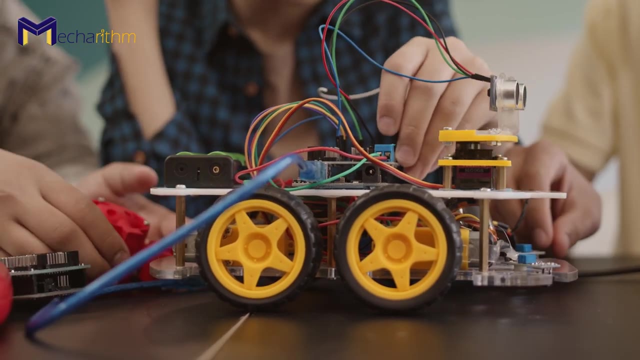 is what exactly do mechatronics engineers do? Mechatronics system engineers design and select analog and digital circuits, microprocessor-based components, mechanical devices, sensors, actuators and controls, so that the final product meets a specified goal, For example. 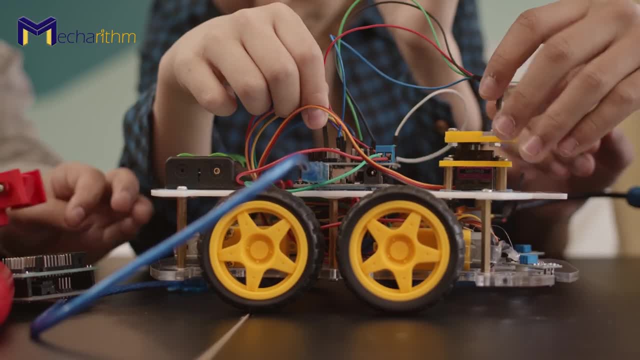 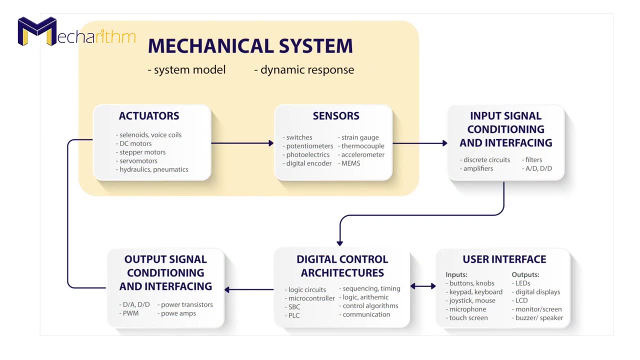 for this mobile robot. it can be programmed to follow a specified path. Let's now take a look at the main components of a mechatronic system. this figure shows the main components of a mechatronic system. motion or action is produced by actuators. sensors detect the state of system, parameters, inputs and outputs for 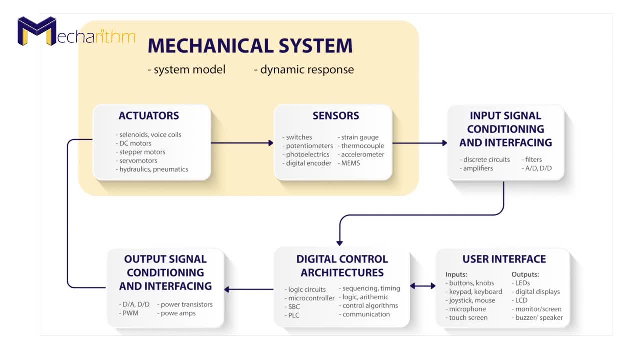 example, a sensor can measure the position or velocity of the motor. this signal is then given to the control system after conditioning. the conditioning and interfacing circuits connect the control circuits with the input-output devices. the control system inputs the control signal and the actuator motion can be controlled accordingly. the user interface enables: 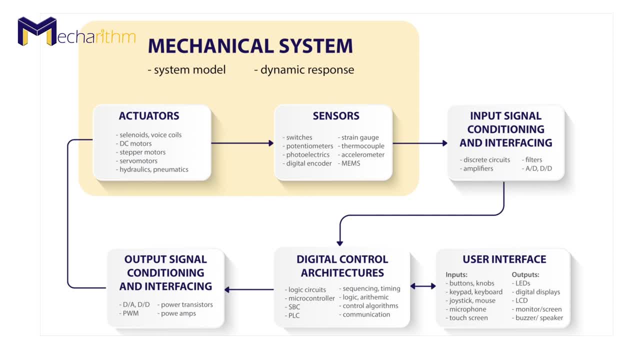 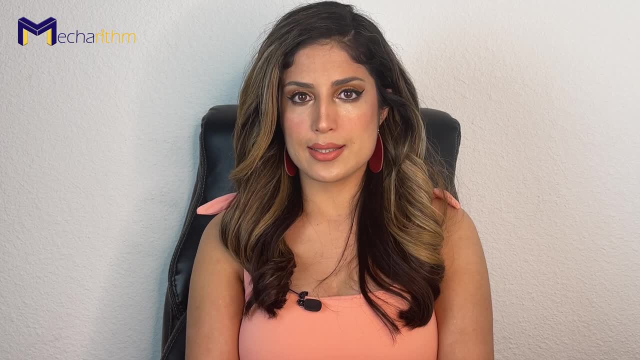 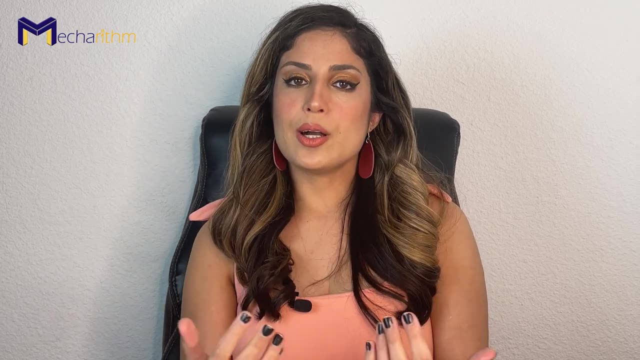 manual inputs and provides graphical displays or visual feedback. the diagram was intended to convey the overall idea of the main components of a mechatronic system. we'll examine each component with lots of practical examples in greater details at the coming lessons, but for now just keep watching until the end of the video. 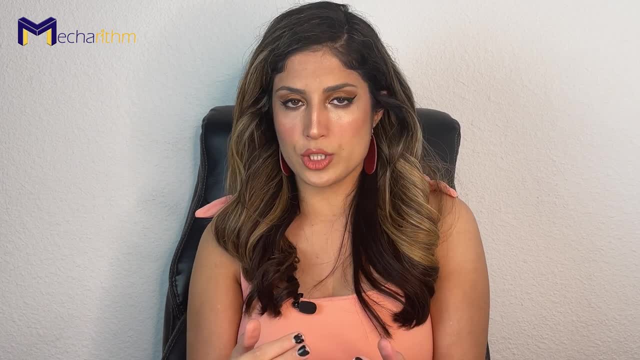 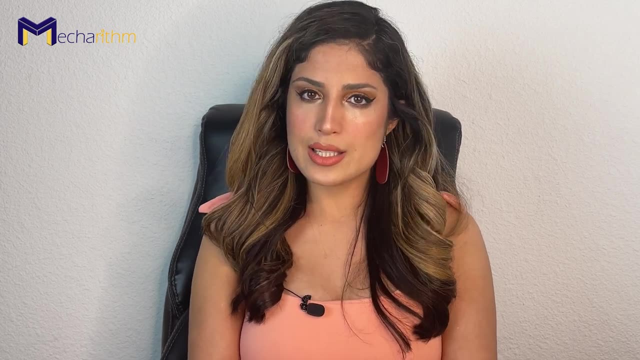 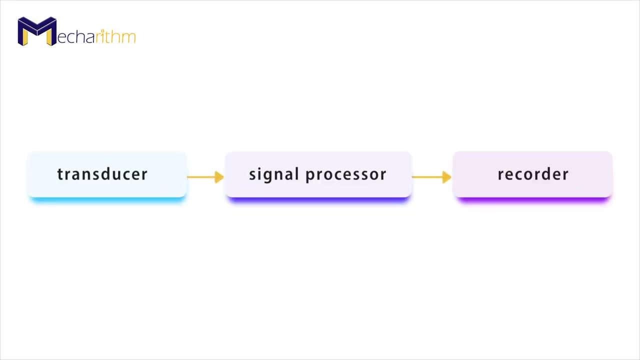 get a visual understanding of how these components are related to each other in a mechatronic system. a fundamental part of many mechatronic system is the measurement system. let's see what the elements of a measurement system are. this figure shows the elements of a measurement system generally, a. 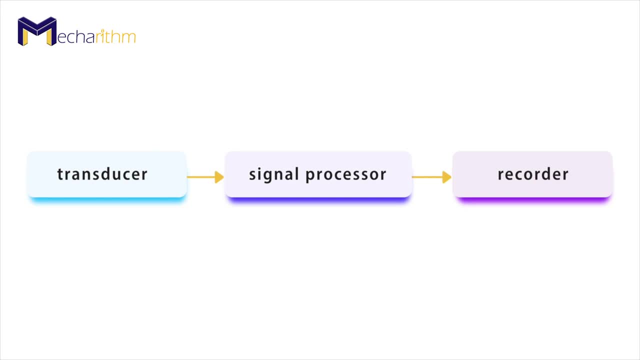 transducer is a sensing element that converts a physical input into an output, which, which is usually a voltage. a signal processor performs filtering, amplification or other signal conditioning on the transducer output. a recorder is an instrument, a computer or an output device that stores or displays. 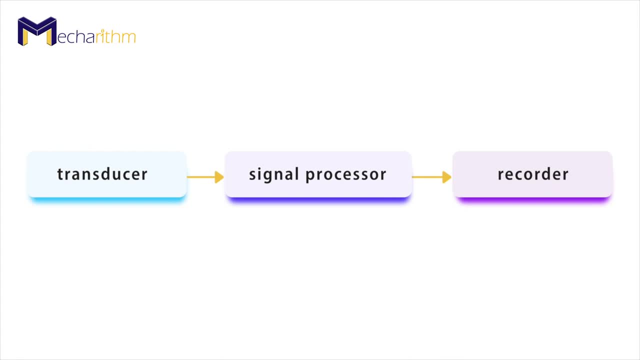 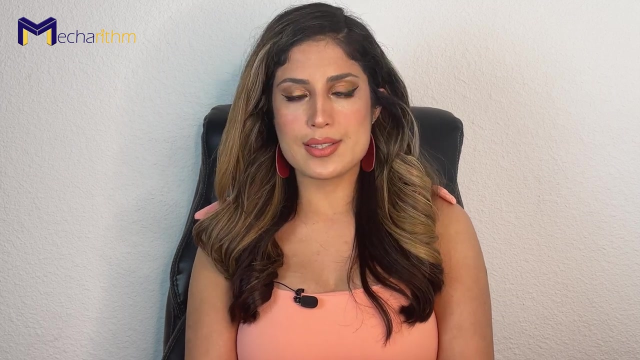 sensor data for monitoring or subsequent analysis. the term sensor refers either to the transducer or the combination of the transducer and the signal processor. let's now see an example of a mechatronic system with all the components that we discussed. a robot vacuum cleaner is an autonomous machine that 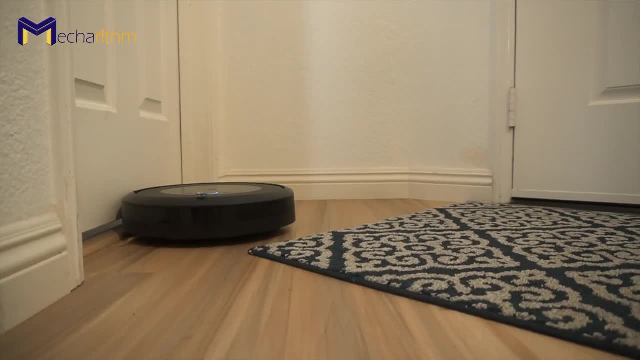 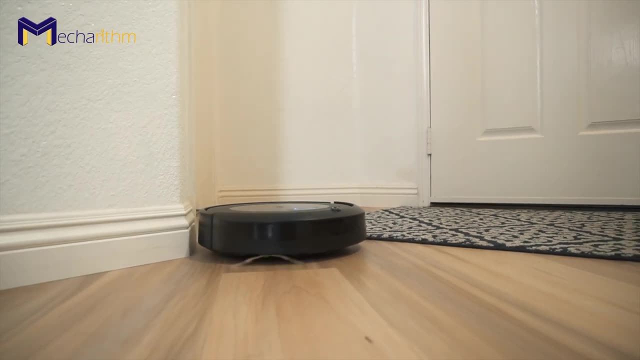 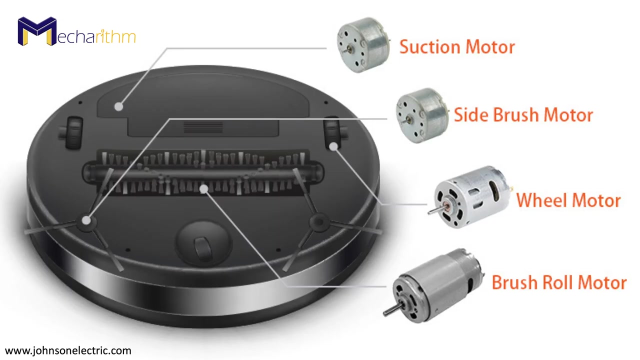 automatically maneuvers itself around the room. to clean it, a spinning brush and a vacuum are used to pick up dirt. as with a conventional cleaner, the two large wheels are driven independently by two separate electric motors. it can also have other actuators, like a suction motor, side brush motor or brush roll motor. the 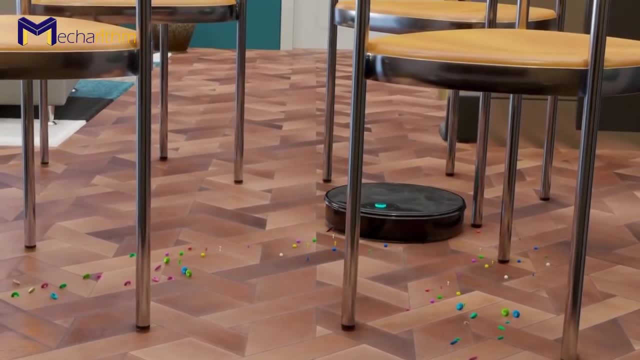 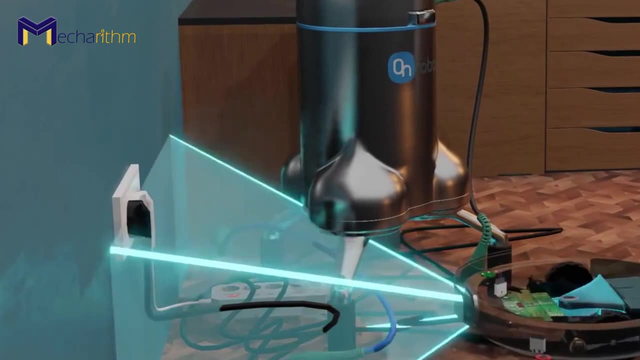 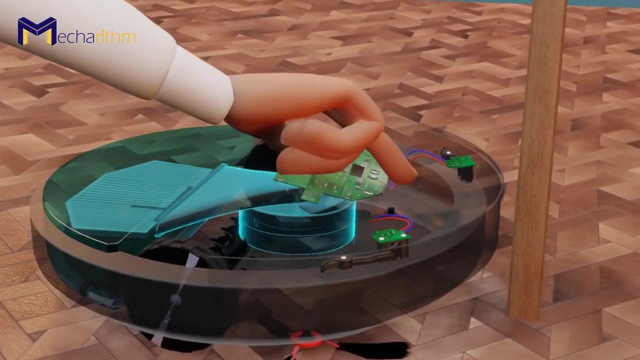 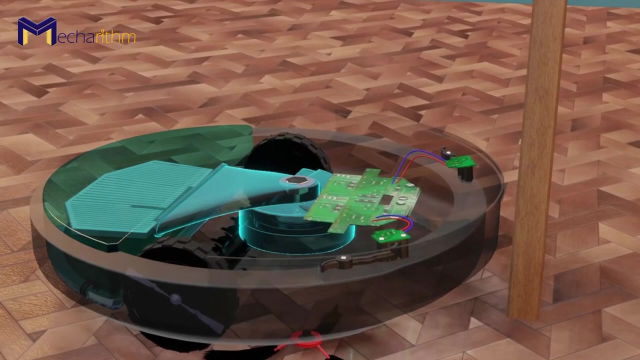 different onward sensors enable the robot vacuum cleaner to move autonomously, detecting dirt, avoiding obstacles and avoiding things like tassels on rocks and telephone cords. sensors can detect walls and obstacles, then send signals to the control unit so the robotic vacuum cleaner slows down or changes direction. furthermore, stairs and deep drops can be detected by sensors.